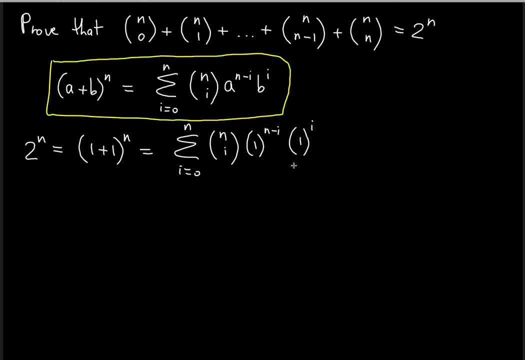 1 raised to the i. Okay, And now we can express that as: starting from the 0 for the i, for the first i equal to 0. So we're going to have n, choose 0. And then we're going to have: 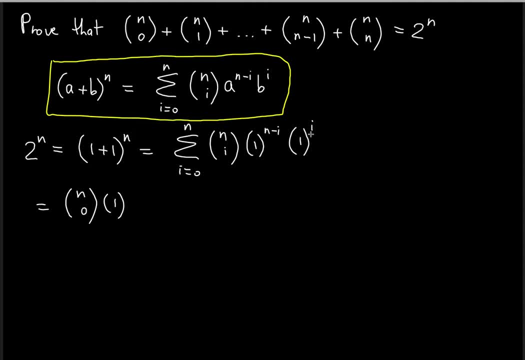 1 to the n minus 0, because i is equal to 0.. So it's just n, Okay, And well, I will just write it like that. So just so you know what I'm substituting. And then another 1. 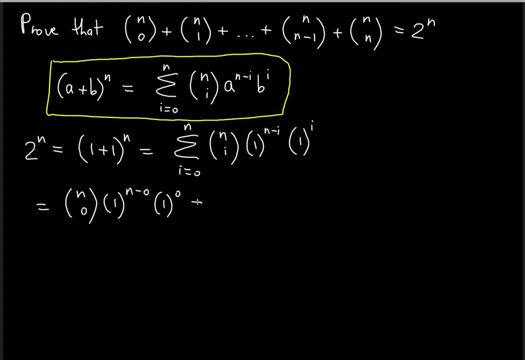 by i is 0.. So to the 0 plus another 1.. The next one is going to be n choose 1, because that's the next. i right, We're going in whole numbers, counting numbers: n choose 1.. And then 1 raised to the n minus 1 times 1, to the first power, etc. Until the. 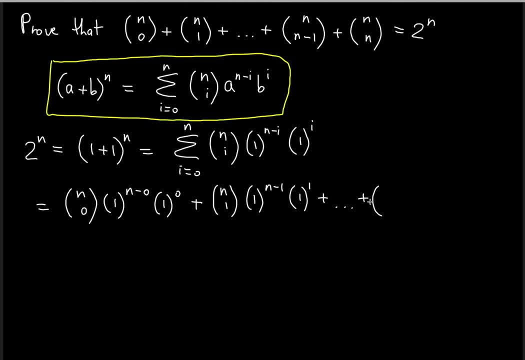 very last two terms. The very last two terms will be what It will be: n choose n minus 1.. Okay, And then we're going to have 1 to the n minus n minus 1.. And then we're going to have 1 to the n minus n minus 1, right. n minus n minus 1, right, And then another. 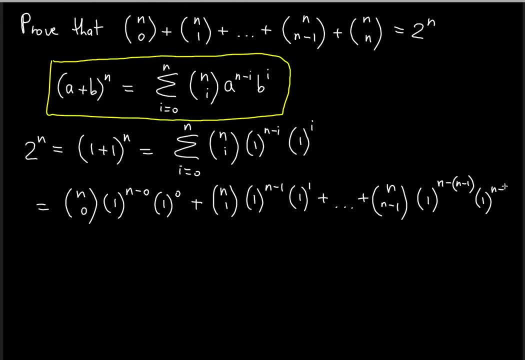 one by n minus 1, right n minus 1.. And then the last term will be what It will be: n choose n. of course, That's when the i will reach the n. So n choose n, And then 1 times n minus. 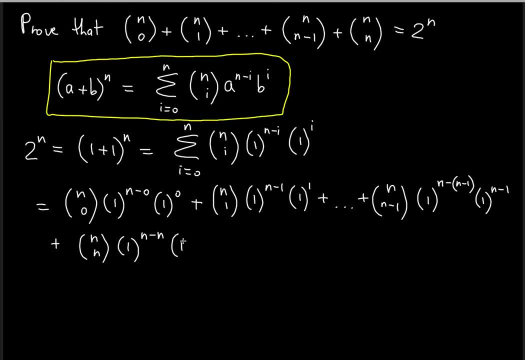 n right The top minus the bottom Times 1 to the raised to the bottom, only right. So what is that? equal to Notice n choose, 0 is 1.. So that's 1. And 1 raised to the nth. 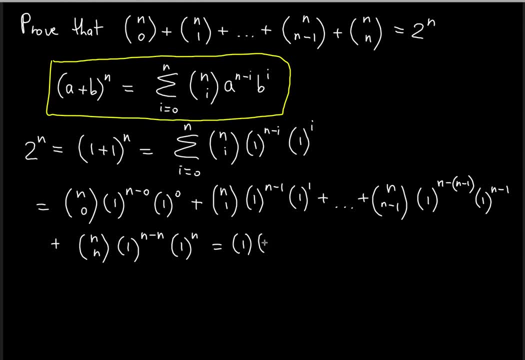 power is still 1.. n minus 0 is n 1, raised to the n is still 1.. And then 1 to the 0, power is still 1 as well. And then we're going to have n choose 1, right n choose 1.. And by: 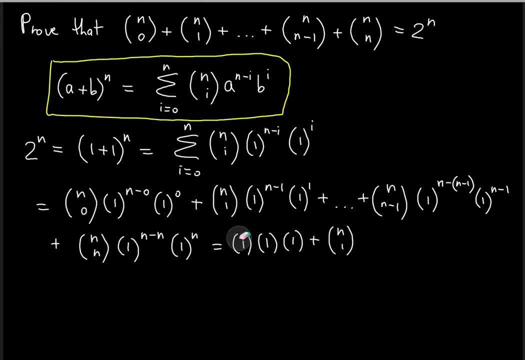 the way I want to leave. I want to leave n choose 0 the way it is, because that's what we want to show on the left side. So I'm going to just write n choose 0.. I'm going to leave it as it is, Even though 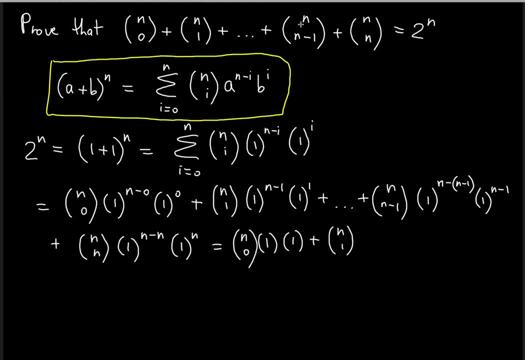 I know n choose 0 is 1, but I'm just going to leave it as it is for the sake of showing the left side of this equation that we need to use for proof. So that's that. And then n choose 1 is going to be what n choose 1.. 1 to the n minus 1 is still 1.. 1 to the 1. 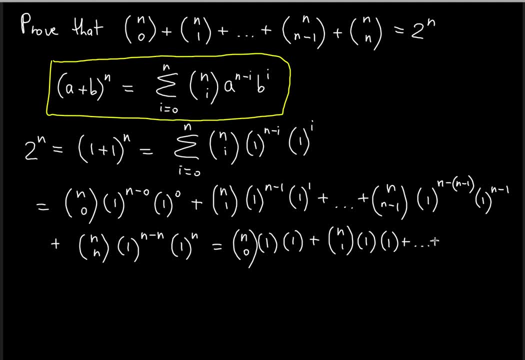 is still 1, etc. Until we get n to the n minus 1.. n choose n minus 1.. Everything else is 1, right 1 raised to pretty much any whole number is still 1.. That doesn't change. This is still. 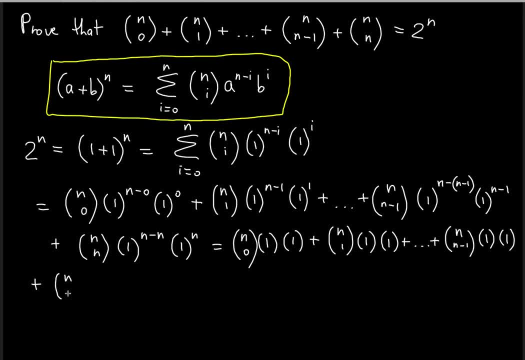 1.. And then the last term is n, choose n. And again, 1 to the 0 is still 1.. 1 to the n is still 1.. So what do we get as a result? We get n choose 0..